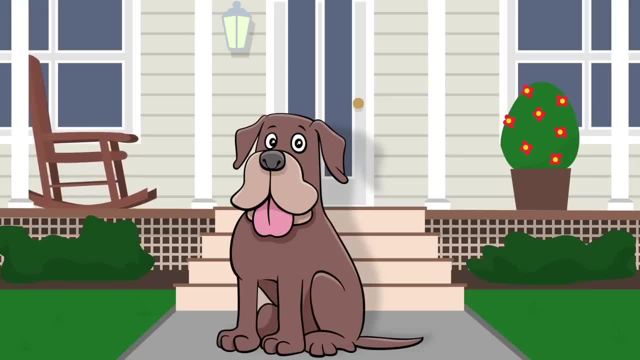 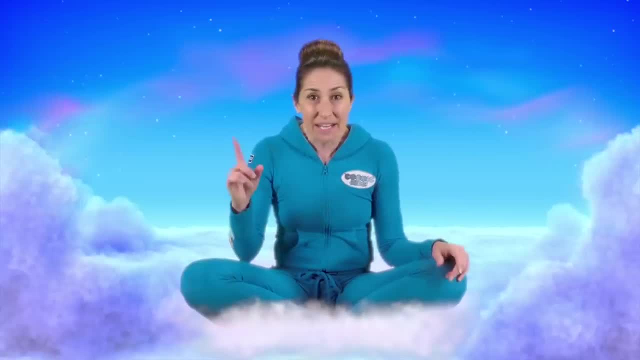 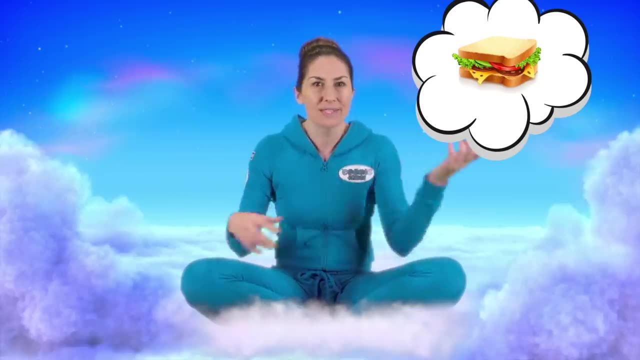 thing we were focusing on, Just like a dog who goes from thinking ball, then bone, then squirrel, all in the space of five seconds, One minute. we're focused on our breathing. The next we're thinking about what's for dinner and about something someone said at. 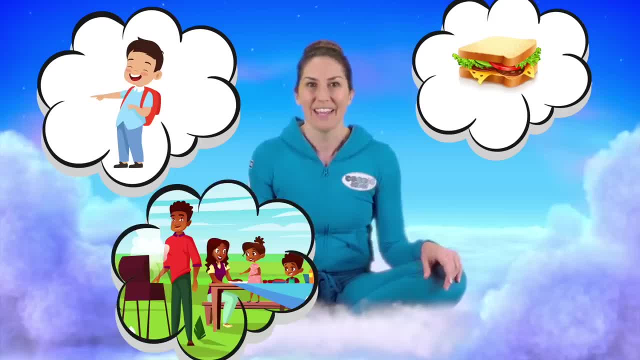 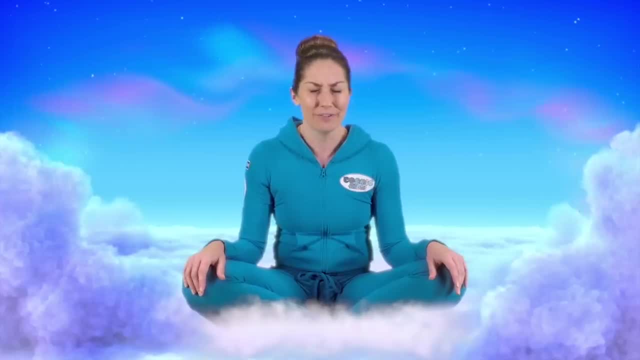 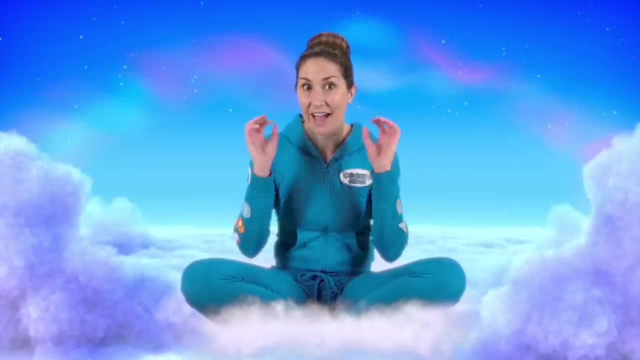 school today, then about how much we're looking forward to the weekend, then about our favourite TV show, then about, oh, just so many thoughts And it's just not very relaxing. When we practice mindfulness, we are training our mind to be better at focusing and choosing. 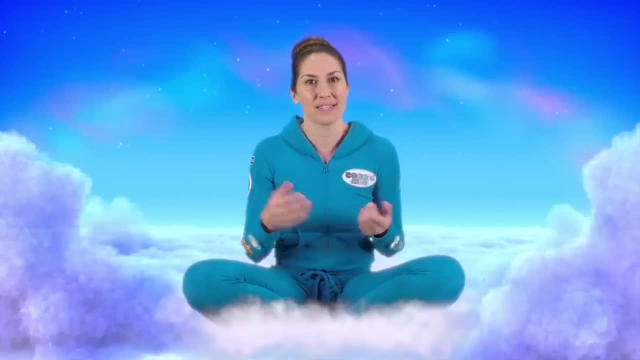 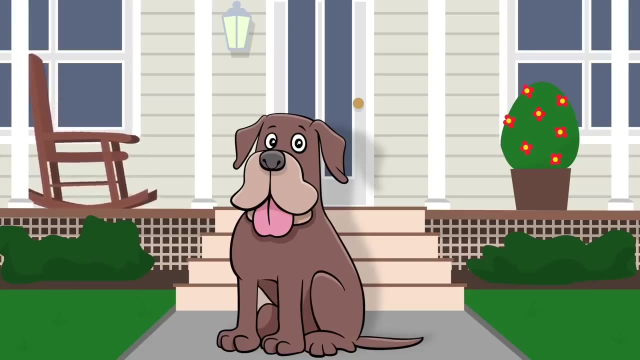 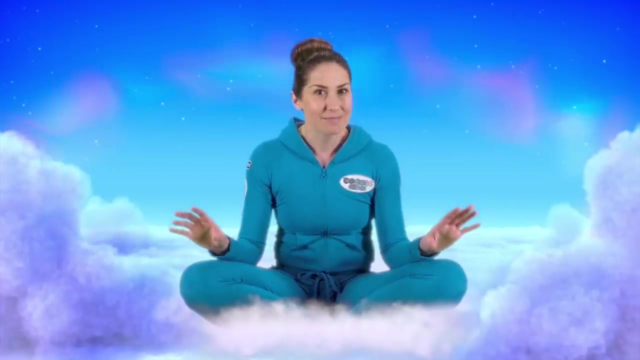 which thoughts we want to act on or let pass. We want that dog to slow down and to settle on one thing for a bit longer, And the great thing is this will make us feel more calm and relaxed, which is amazing. It's lovely. 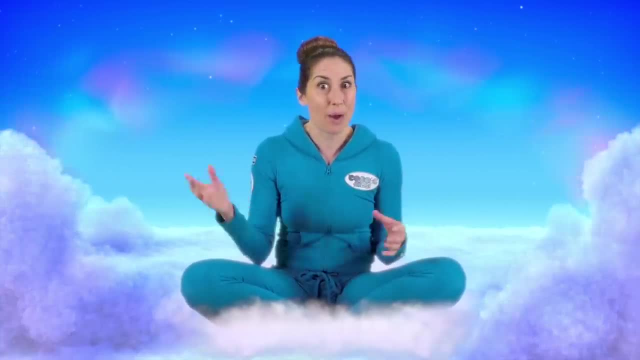 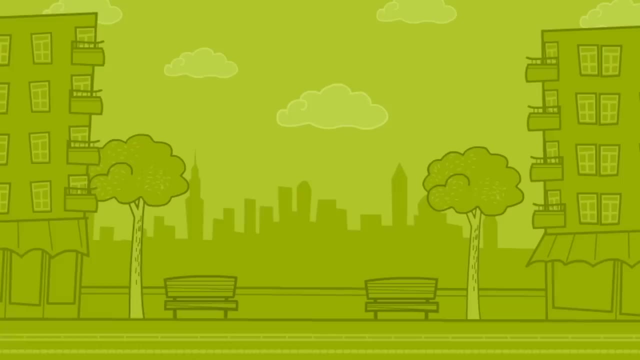 When I practice, I can almost see my thoughts passing and I can choose which ones to act on and which to leave alone and let go. It's like I'm standing on the side of a road watching buses going past. These are my thoughts And I can decide which ones I want to ride and. 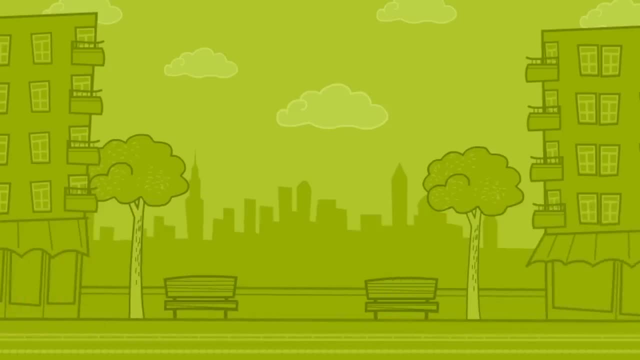 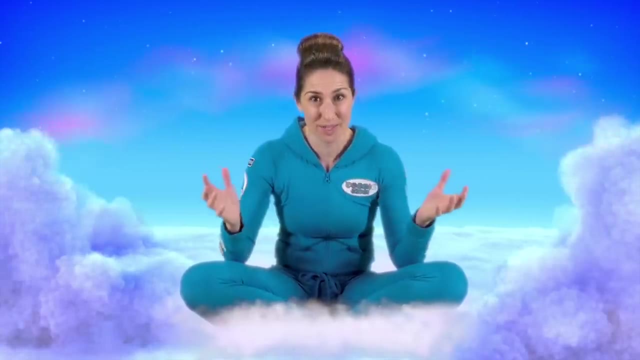 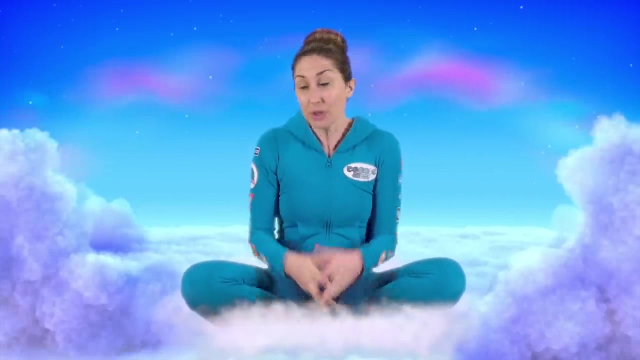 which aren't going my way. We only get to know our mind, though, when we spend time with it, And that is what our mindfulness practice is. Okay, so here's how I practice mindfulness. You can call it meditation if you like, They're. 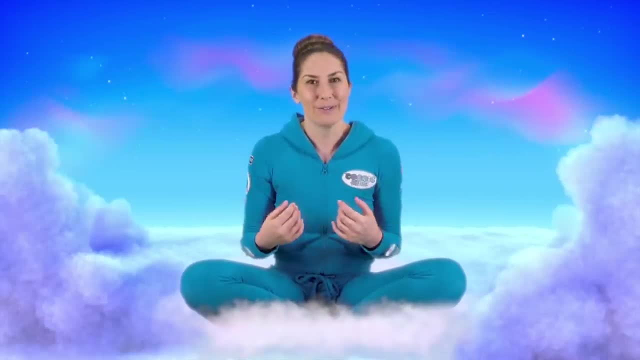 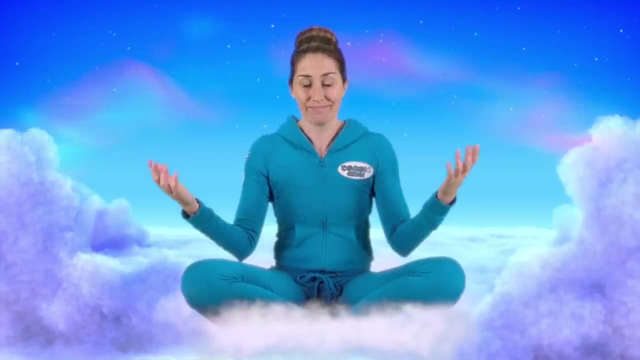 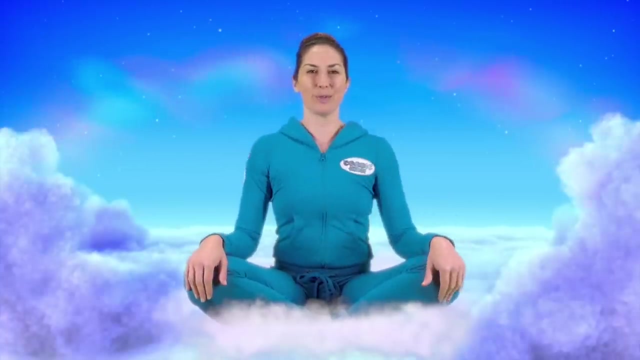 both the same thing, really. I'll explain what I do and if you listen carefully you'll learn what I do and you can try it yourself whenever you like. Okay, here's how it works. Posture: I find it easiest if I sit with a nice tall spine, like I'm sitting on a 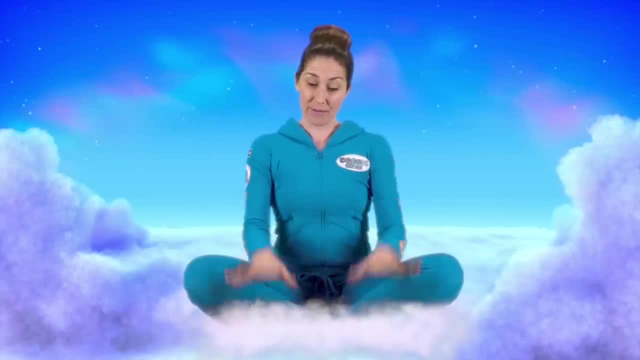 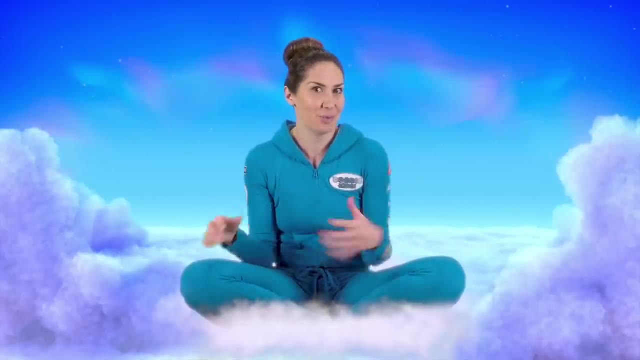 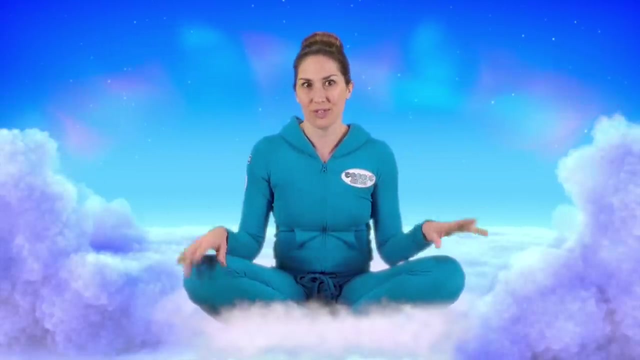 throne like a king or queen, with either both feet on the floor or sitting with my legs crossed. A slouchy posture makes it hard for me to pay attention. well, My eyes? I like to close mine. Our eyes can be a window for all sorts of things that make. 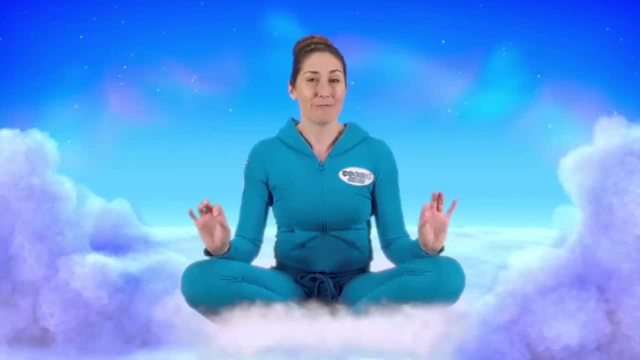 our mind busier with thoughts, So I find it really helps. I can work with my body from any mobility to the most serious kind. I just can't wait the moment I can find- My hands. I try and keep my hands still and rest them on my knees or in my ab. 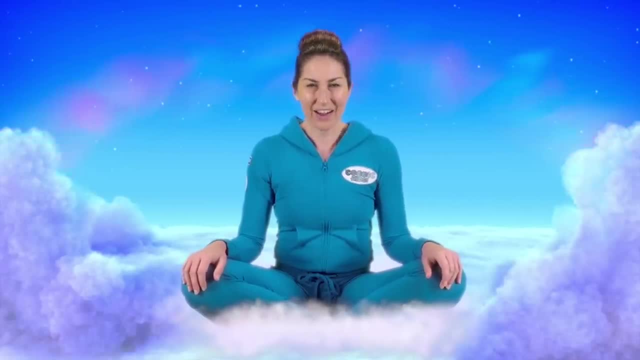 Deep breaths. I take three big filling-up breathes into the chest and out through the mouth. Now I just notice As I sit for a few moments. I focus on my breath coming in, breaking down and applying pressure on the chest. Hi-oh, Hi, Hi, Hi, Hi, Hi, Hi, Hi, Ha, Hi. 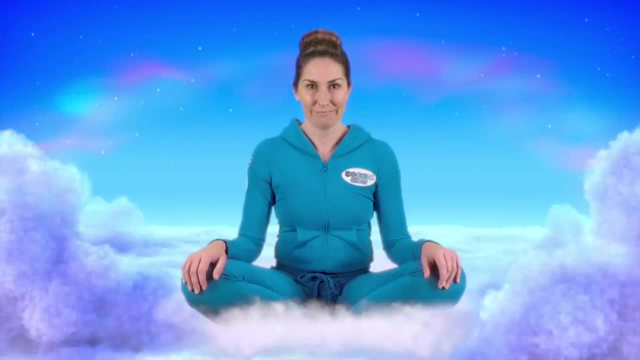 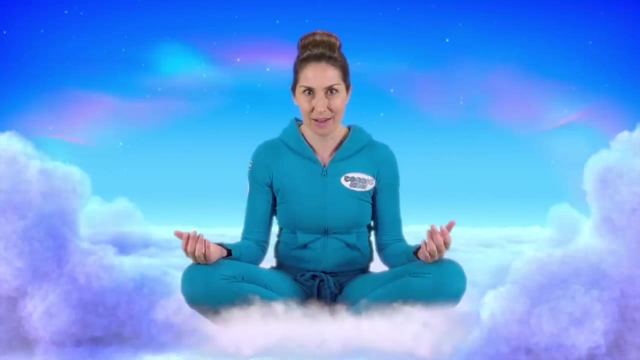 Coming in and going out, And that's it. Now please remember to be kind to yourself and curious. We are interested to see what we notice And we don't judge ourselves as bad or good if our mind keeps jumping about like the little dog, jumping around from thought to thought. 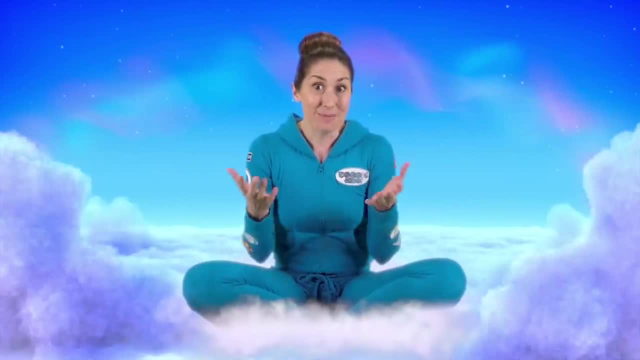 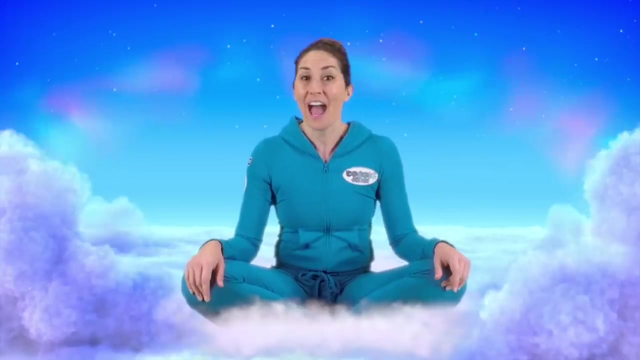 It is what it is. If we manage to keep noticing it and bringing it back, then great. Now practice. It's good to try and do this for a few minutes at the same time every day. This is how you build a strong and connected relationship with your mind. 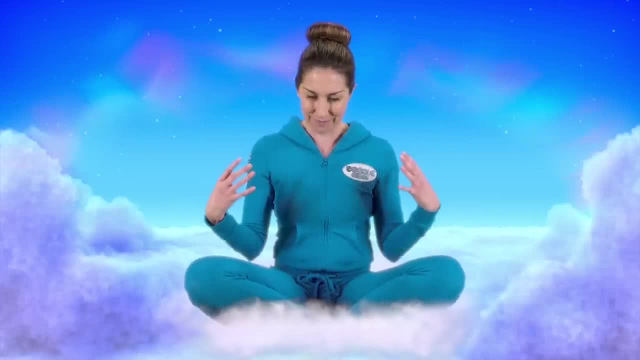 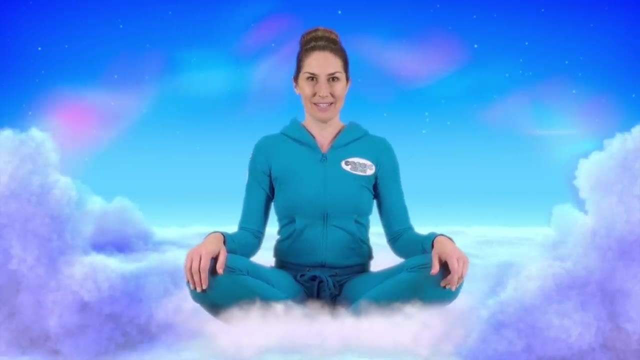 So just to recap Posture: Sitting nice and tall like a king or queen, Keeping our hands nice and still Closing our eyes And taking three deep breaths in through our nose and out through our mouth. Then we notice Watching our breath coming in and going out. 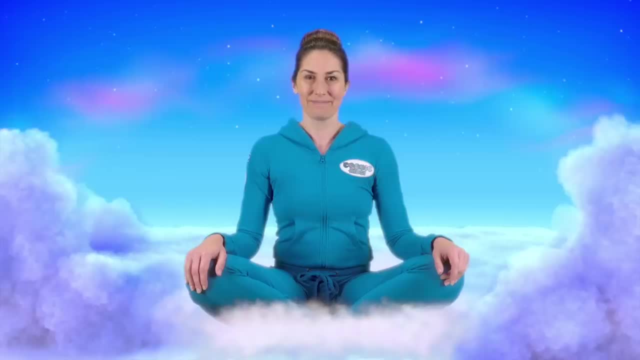 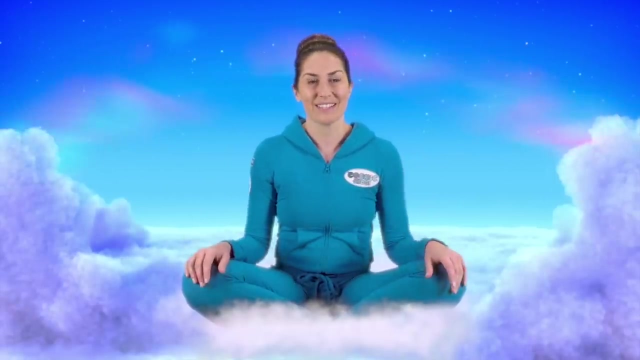 Coming in and going out. I like to do my mindfulness practice each morning for five minutes. I find that when I do this I'm much calmer in the day And I'm better at learning things and dealing with whatever comes up that day. 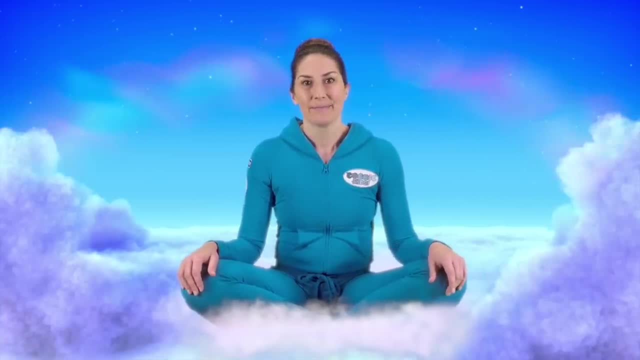 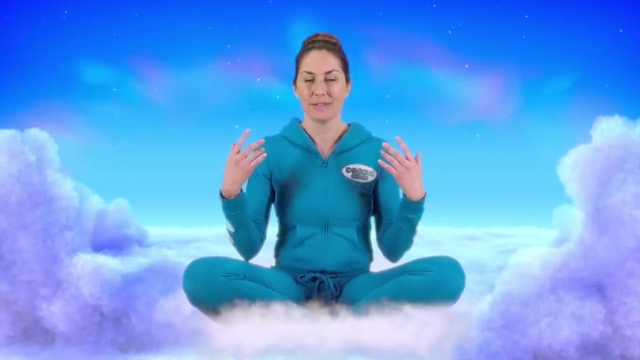 I also do it at night when I'm going to sleep. Sometimes my mind will still be busy with thoughts and I need to settle it down a bit. So I lie in bed, close my eyes and focus on the breath coming in through my nose and out through my mouth.